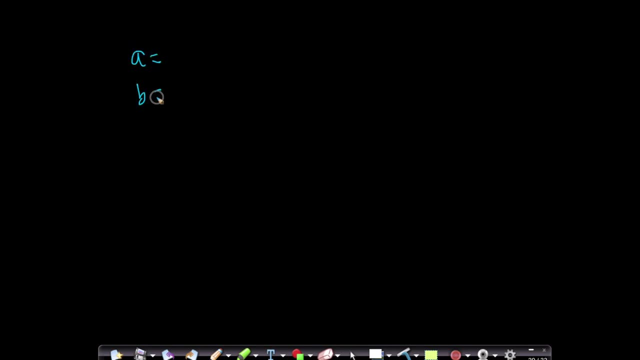 So imagine if you are given two vectors, A and B. Let us assume both of them are row vectors. Let us assume I have A1, A2, so on, so forth. AN. Similarly vector B, which has B1, components B1,. 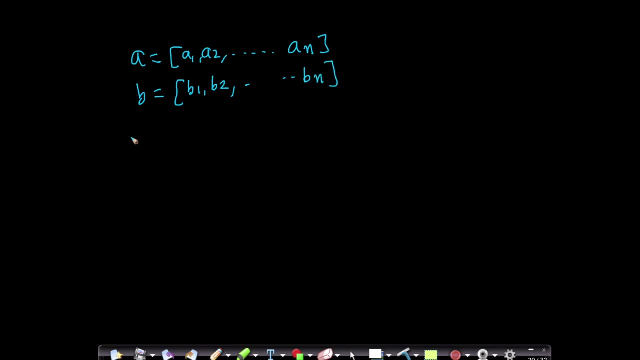 B2, so on, so forth, BN. Now, mathematically, let us learn some very basic operations. What about addition of A and B? If I add these two vectors, what do I get? I simply get. it is basically called component wise addition A2 plus B2.. So what I am doing here is: I am basically taking 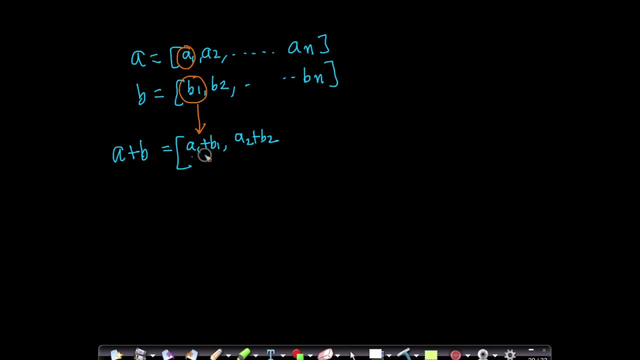 the first component from both A and B and I am summing it up, That becomes the first component of A plus B. Let us assume A plus B equals to C. Similarly, I am taking the second component here and I am summing it up here. Very, very straightforward idea. So, so on, so forth. 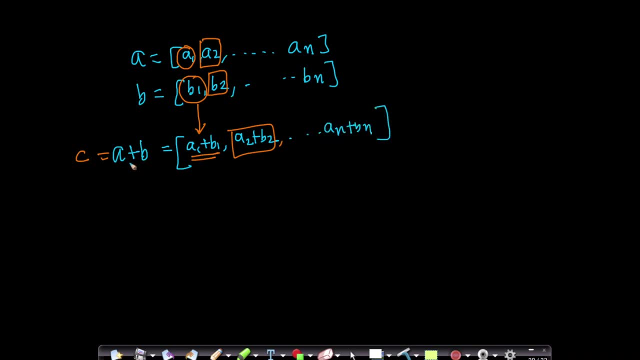 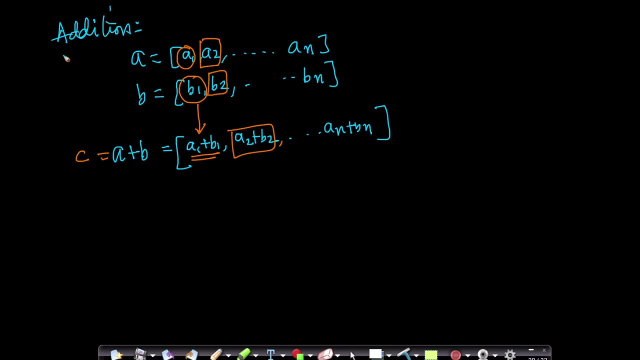 the addition of vectors. Then the immediate question that comes to your mind is: is there something like multiplication? Because we learned all these concepts in simple algebra, right? So is there a concept of multiplication of two vectors? There are actually for vectors. 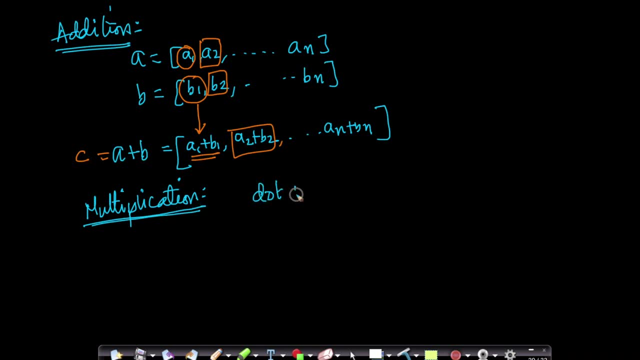 there are two types of multiplications. There is something called a dot product and a cross product. There are two types of multiplications, So some of you who have studied physics in your 11th and 12th grades would recall what a dot product is and what a cross product is. 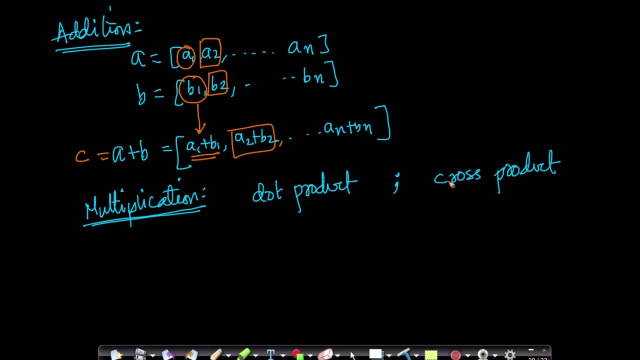 So just for simplicity, we do not use cross product much in machine learning, So I will not go into the details of what a cross product is. But let us go and understand what a dot product is. So if I am given two vectors, A and B, a dot product is written as A dot B. First I will 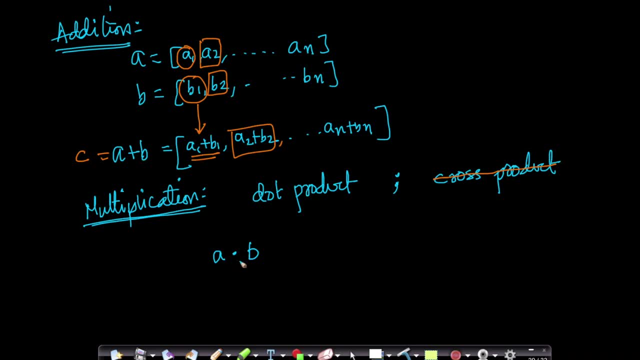 explain the notation and then we will go and understand the geometry behind it. So A dot B is nothing. but you take again, it is a complex product. So you take again, it is a complex product. So A dot B is nothing but A1 multiplied by B1 plus A2, multiplied by B2 plus A3, multiplied by B3,. 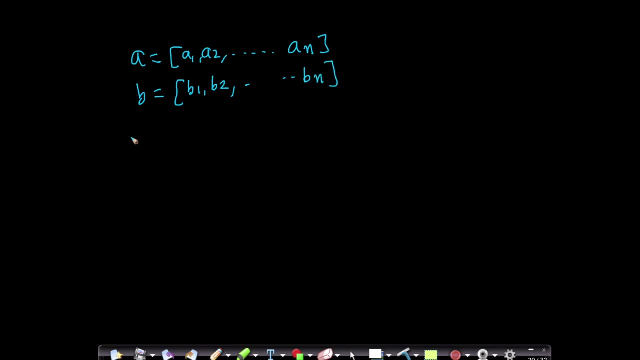 B2, so on, so forth- BN. Now, mathematically, let us learn some very basic operations. What about addition of A and B? If I add these two vectors, what do I get? I simply get. it is basically called component-wise addition: A2 plus B2.. So what I am doing here is: I am basically taking 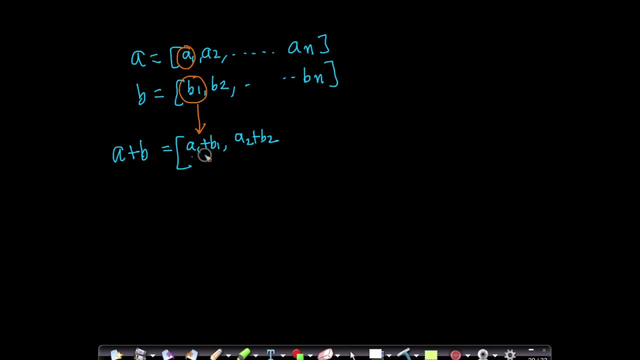 the first component from both A and B and I am summing it up, That becomes the first component of A plus B. Let us assume A plus B equals to C. Similarly, I am taking the second component here and I am summing it up here. Very, very straightforward idea. So, so on, so forth. 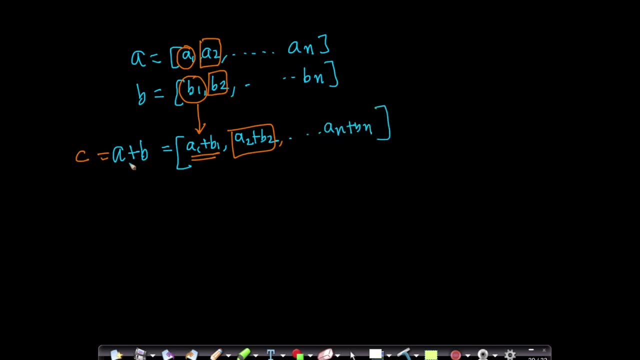 AN plus BN. This is how you add two vectors. Very, very simple idea. This is the way to do it. So let us assume A plus B equals to C. So let us assume A plus B equals to C- The addition of vectors. Then the immediate question that comes to your mind is: 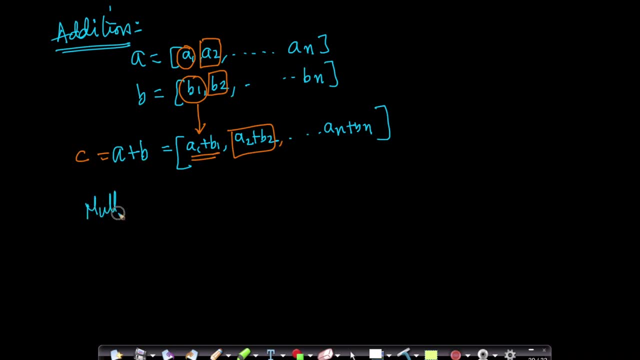 is there something like multiplication? Because we learned all these concepts in simple algebra, right? So is there a concept of multiplication of two vectors? There are actually, for vectors, there are two types of multiplications. There is something called a dot product. 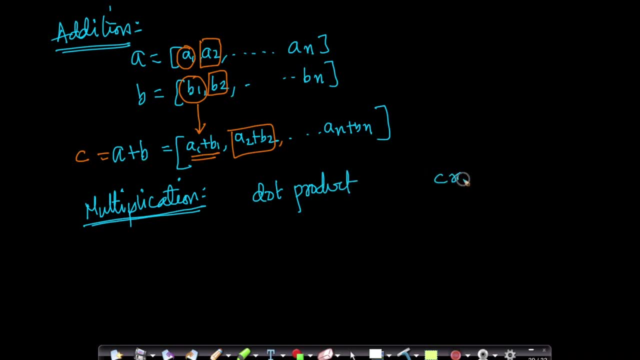 and a cross product. There are two types of multiplications, So some of you who have studied physics in your 11th and 12th grades would recall what a dot product is and what a cross product is. So, just for simplicity, we do not use cross product much in machine learning, So I will not. 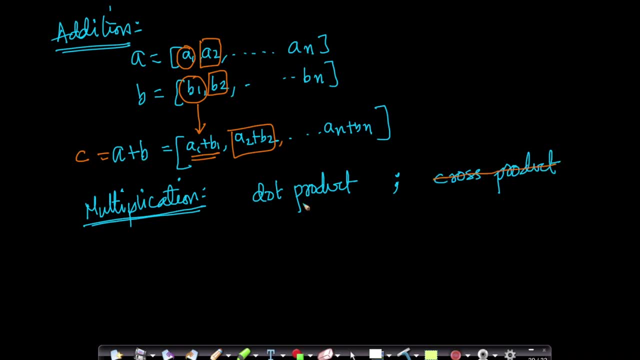 go into the details of what a cross product is, But let us go and understand what a dot product is. So if I am given two vectors, A and B, a dot product is written as A dot B. First I will explain the notation and then we will go and understand the geometry behind it. So A dot B. 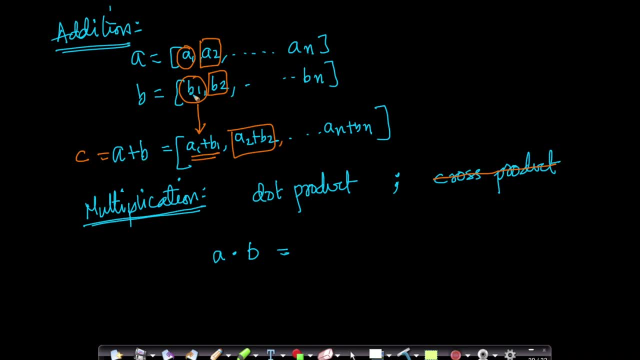 is nothing. but you take again, it is a complex product. So you take A dot B and you take A dot B. It is a component, wise multiplication. A dot B is nothing but A1 multiplied by B1 plus A2 multiplied. 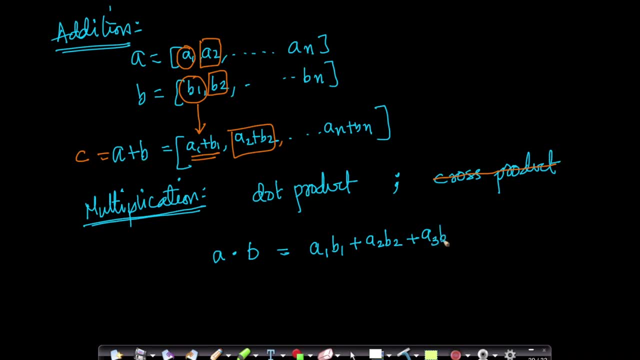 by B2 plus A3 multiplied by B3, so on, so forth. AN multiplied by BN, You might ask: okay, this multiplication part seems logical to us, but why are you adding? Just take it from me that this is just notation. Okay, just let us assume we are understanding notation. I promise you I will. 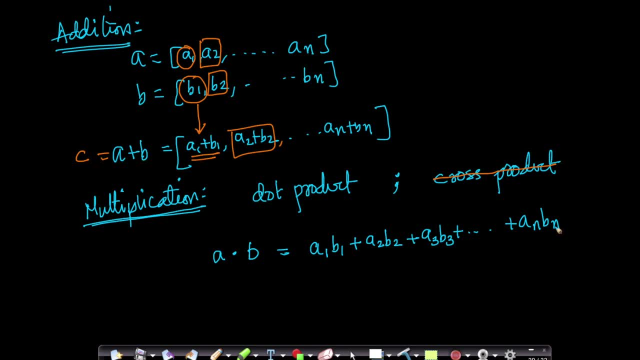 so on, so forth. AN multiplied by BN, You might ask. okay, this multiplication part seems logical to us, but why are you adding? Just take it from me that this is just notation. okay, Just let us assume we are understanding notation. I promise you I will connect it with geometry very. 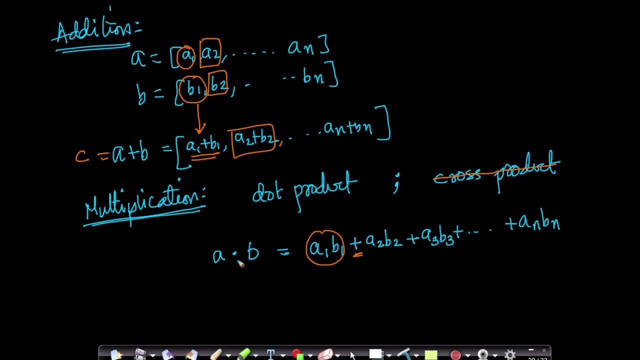 very soon, very quickly, okay. So for now, let us define it this way: Now, if I write it in vector notation, what is this? A1, B1 plus A2, B2, A3, B3, so on, so forth, I can actually write it. 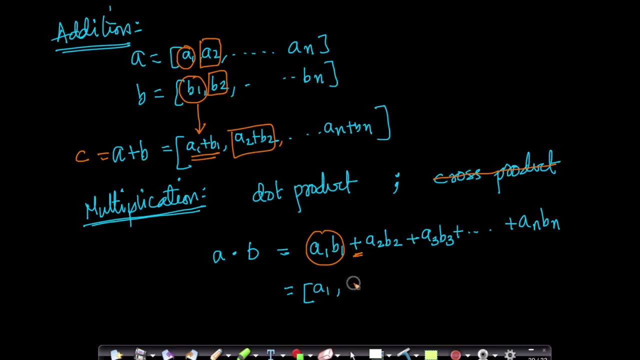 in vector notation. right, I can write it as A1, A2, so on, so forth. If I have a row vector for A and if I have a column vector for B, B1, B2, so on, so forth. BN- some of you might have studied. 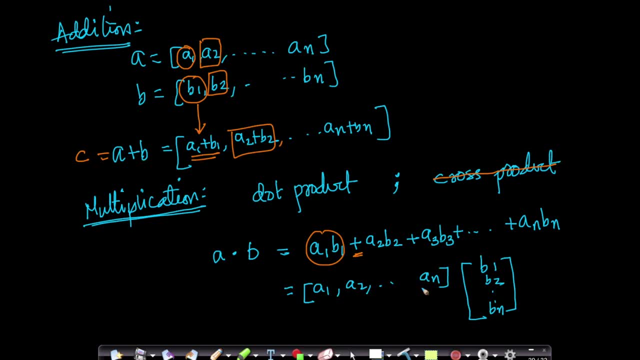 about, about multiplying matrices and multiplying vectors in your 11th or 12th grade. So what does this mean? This basically means that. so this is, first of all, let us remember, this is a 1 cross n matrix or 1 cross. it is basically a row vector. This is a column vector. 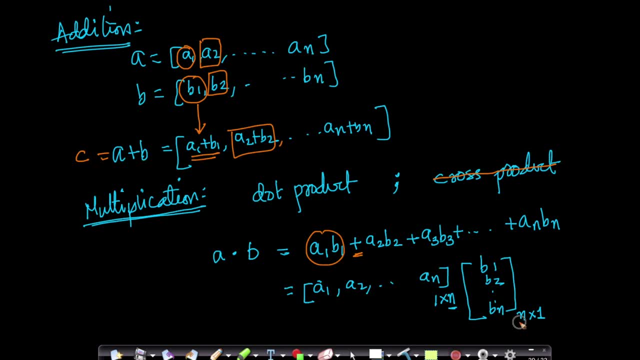 which means it is n cross 1.. As long as this and this match, you can multiply them right? So, since this is n and this is also n, you can multiply these two vectors or these two matrices, if you want to think about it. This is a matrix with only one row. this is a matrix with only one. 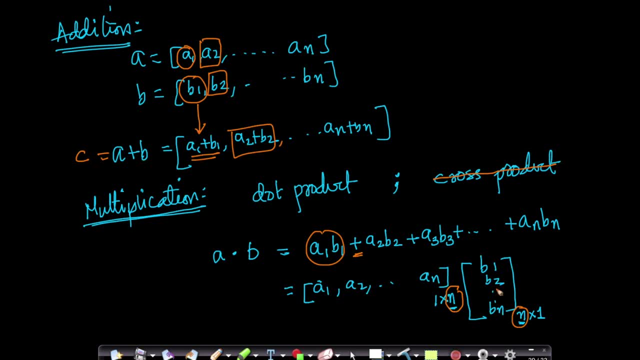 column right. When I multiply them, the simple matrix multiplication that we all learned in high school, it is nothing but a1 multiplied by b1, plus a2 multiplied by b2, and so on and so forth. right Now, from a notation standpoint, typically whenever somebody says a vector, 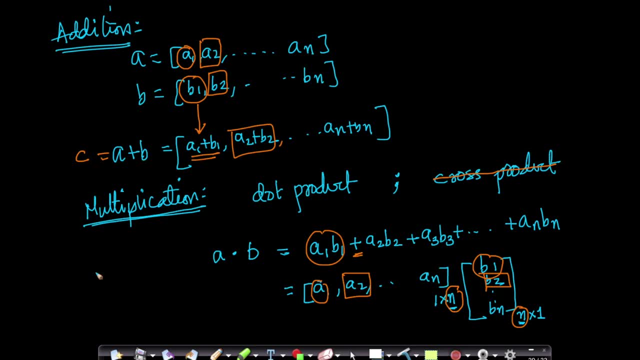 they typically just for notation sake. they typically refer to it as a column vector. So whenever somebody says a is a vector of size n, what do they mean? They typically mean that a is a column vector. This is just for simplicity. 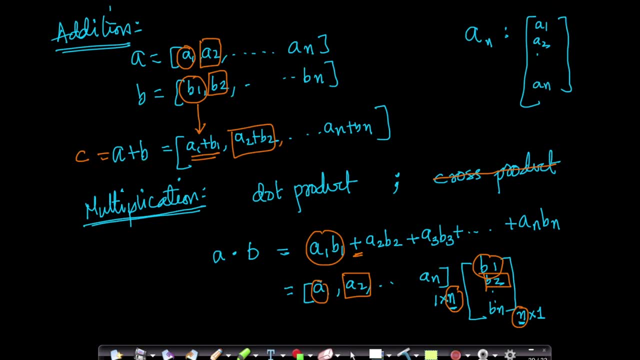 Whenever somebody says a vector, by default it is a column vector. because there is always this confusion: is a given vector column vector or row vector? If nothing is explicitly told about it, you have to assume that it is a row. it is a row, it is a column vector. sorry, right. 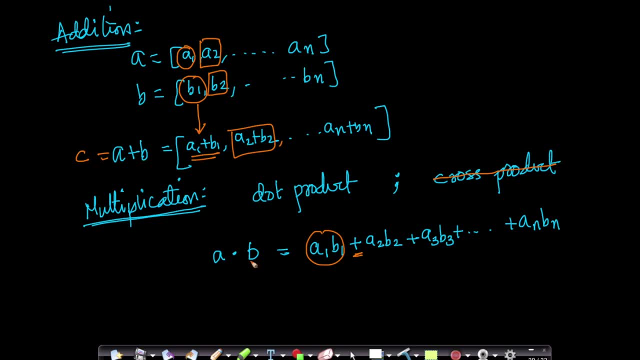 connect it with geometry. So let us assume we are understanding notation. I promise you I will connect it with geometry very soon, very quickly. Okay, So for now let us define it this way: Now, if I write it in vector notation, what is this? A1, B1 plus A2, B2, A3, B3, so on, so forth. I can. 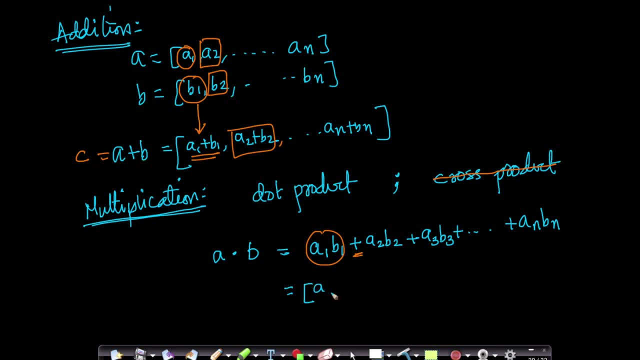 actually write it in vector notation, right? I can write it as A1, A2, so on, so forth. If I have a row vector for A and if I have a column vector for B, B1, B2, so on, so forth. BN, Some of you might have. 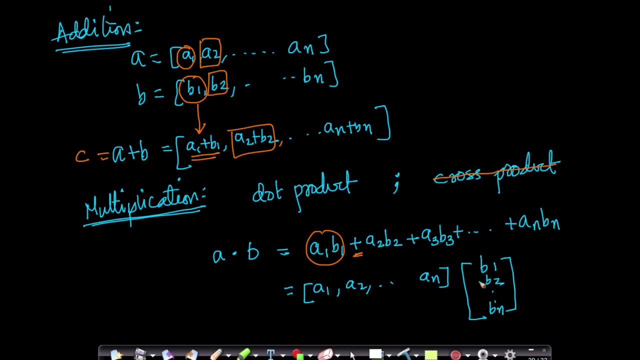 heard about multiplying matrices and multiplying vectors in your 11th or 12th grade. So what does this mean? This basically means that. so this is, first of all, let us remember, this is a 1 cross N matrix or a 1 cross. it is basically a row vector. This is a column vector, which means it: 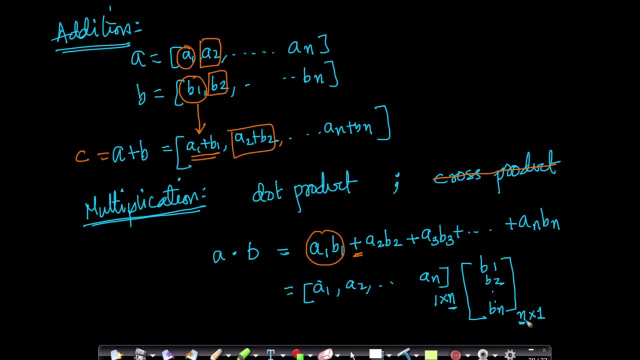 is N cross 1.. As long as this and this match, you can multiply them, right? So since this is N and this is also N, you can multiply these two vectors or these two matrices, if you want to think about it. So this is a 1 cross N matrix or a 1 cross N matrix. So this is a 1 cross N matrix or a 1 cross N matrix. 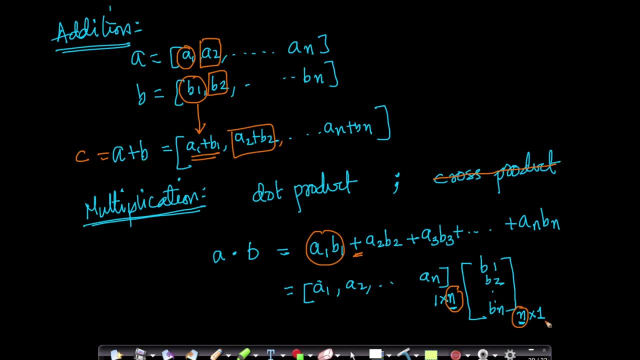 This is a matrix with only one row. this is a matrix with only one column. right, When I multiply them, the simple matrix multiplication that we all learned in high school, it is nothing but A1 multiplied by B1 plus A2 multiplied by B2, and so on, so forth. right Now, from a notation: 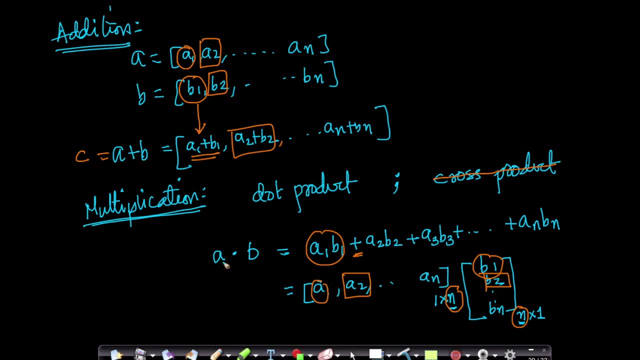 standpoint. typically, whenever somebody says a vector, they typically- just for notation sake- they typically refer to it as a column vector. So whenever somebody says A is a vector of size N, what do they mean? They typically mean that A is a column vector. This is just for simplicity. Whenever somebody 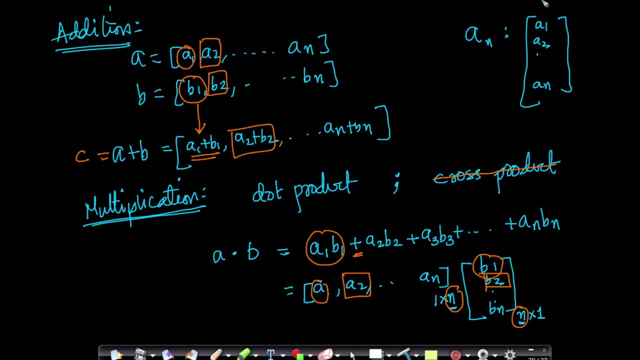 says a vector, by default it is a column vector. Because there is always this confusion: is a given vector a column vector or row vector? If nothing is explicitly told about it, you have to assume that it is a row. it is a row, it is a column vector. sorry. 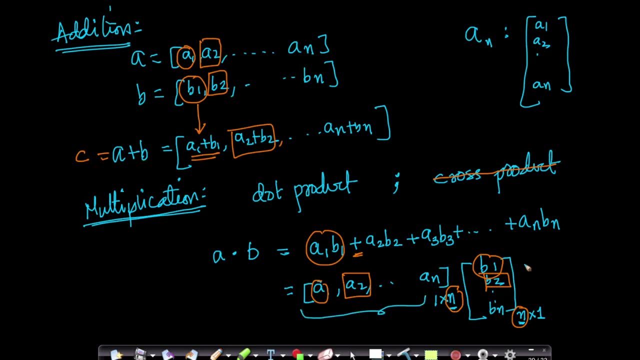 right. So what we have here is a row vector of A and a column vector of B. This is also written as numerically. this is also, I mean for simplicity- when you have a row vector. when you have a row vector, let us assume I have a row vector A1,. 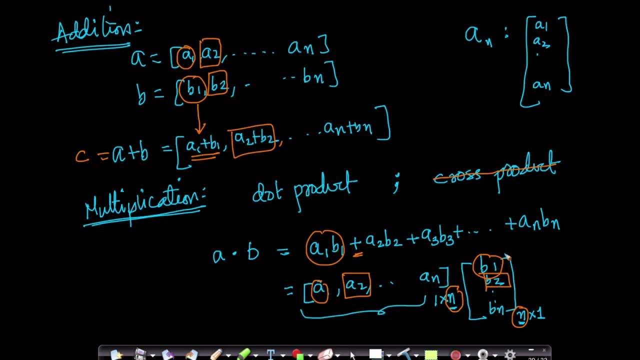 So what we have here is a row vector of a and a column vector of b. This is also written as numerically. this is also, I mean for simplicity, when you have a row vector, when you have a row vector, let us assume I have a row. 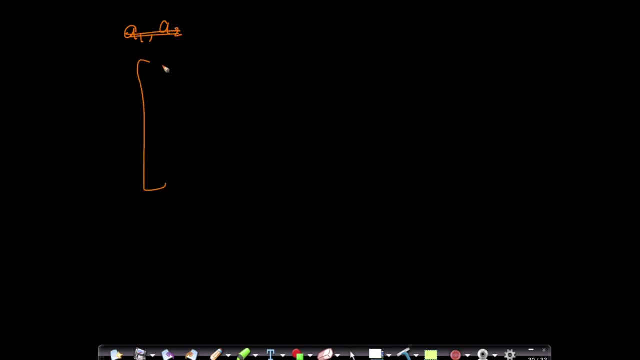 vector a1,. sorry, let us assume I have a column vector. just for simplicity, I have a1, a2, so on and so forth. a n right, Let us assume this is my vector a, because the default representation is: 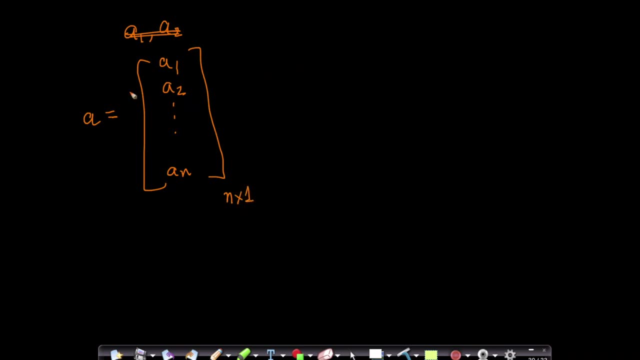 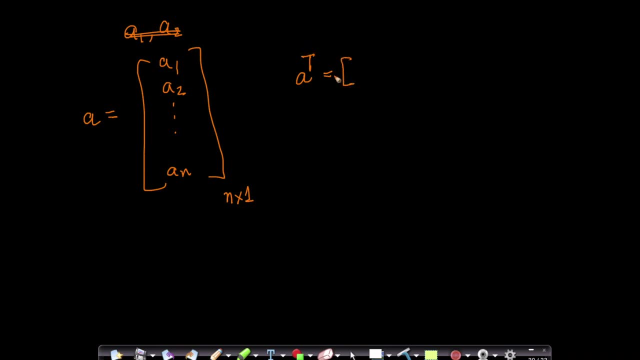 A transpose. for some of you have learned basically in your algebra in your high school or 11th and 12th grade, would immediately recognize this. A transpose is nothing but A1, A2, so on, so forth. A n. 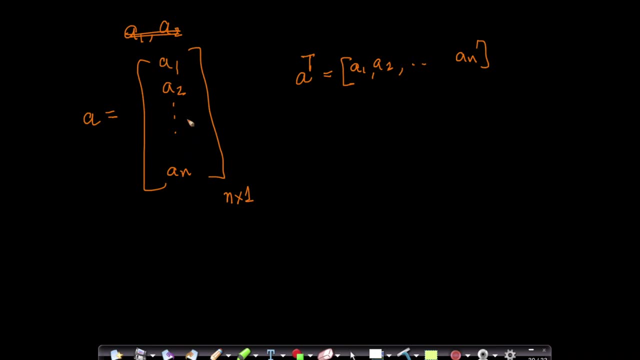 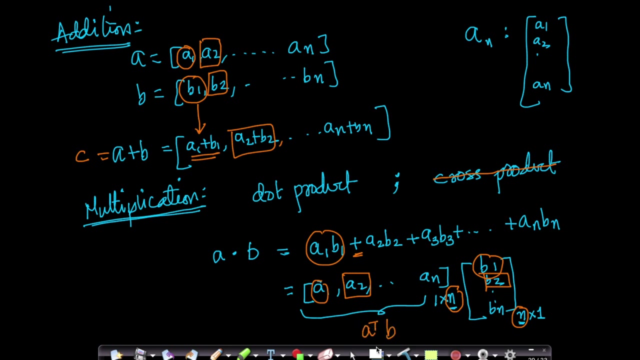 So I can convert a column vector into a row vector by just taking an operator called transpose, and this becomes 1 cross n. So, going back to our previous example, what we have here literally is nothing but A transpose multiplied by B right. 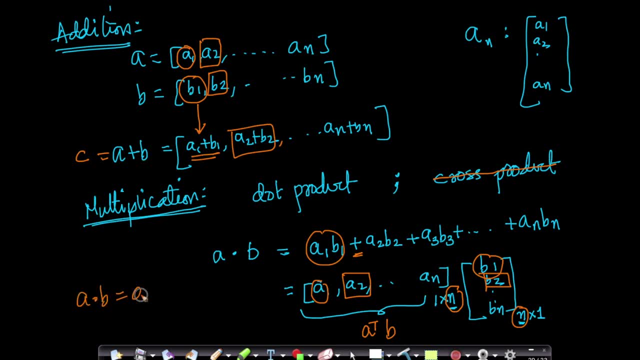 So you can write A dot B as nothing but A transpose B, and what does it all boil down to? It boils down to summation of 1 to n. if A is an n-dimensional vector, A, i, B, i. This is what a dot product is from a pure linear algebraic perspective. 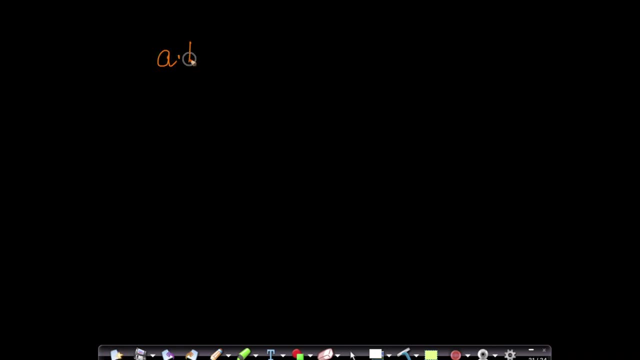 But now let us go and understand geometrically what does A, dot, B mean? because that is important. right, We have to connect geometry with linear algebra, Because if we do not connect it, we do not understand what a dot product means in higher 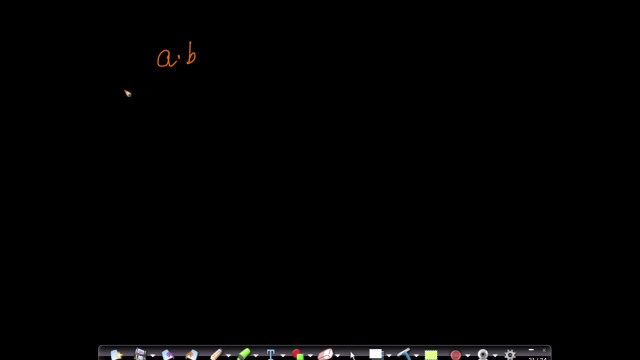 dimensional spaces, Because we are doing all of this linear algebraic exercise to understand geometry. So let us take, let us assume we live in a two-dimensional space or we have a two-dimensional space. Let us assume I have a vector A and I have a vector B. 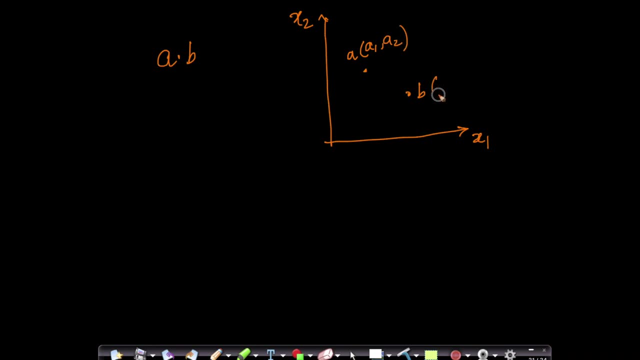 Of course, A has two components: A1 and A2.. B also has two components: B1 and B2, right Now, when we have these two components, this is your vector A, This is your vector B. Now, what does A dot B represent geometrically? 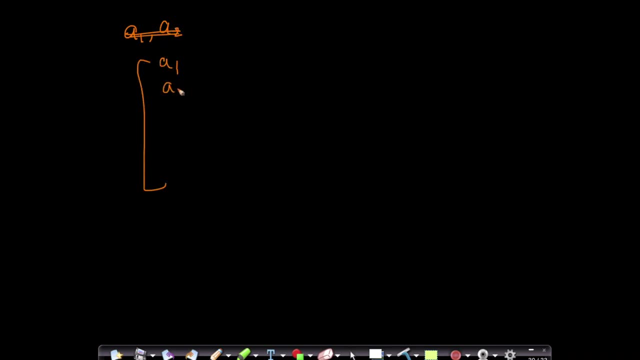 sorry. let us assume I have a column vector, just for simplicity. I have A1, A2, so on, so forth: A1, right. Let us assume this is my vector A, because the default representation is always a column vector which is of size N, cross 1, right, N rows and one column right. 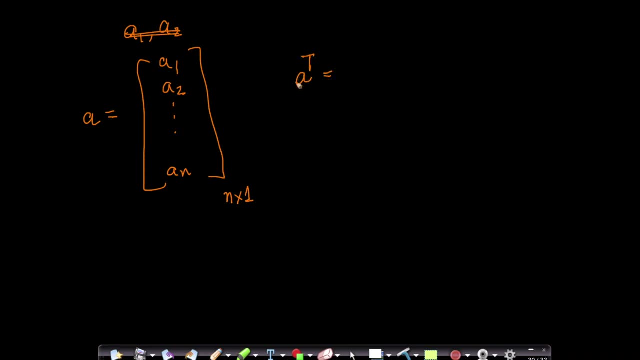 Now, what does A transpose mean? A transpose means basically swap your rows with columns and columns with rows. So A transpose for some of you have learned basically in your algebra in your high school or 11th and 12th grade. 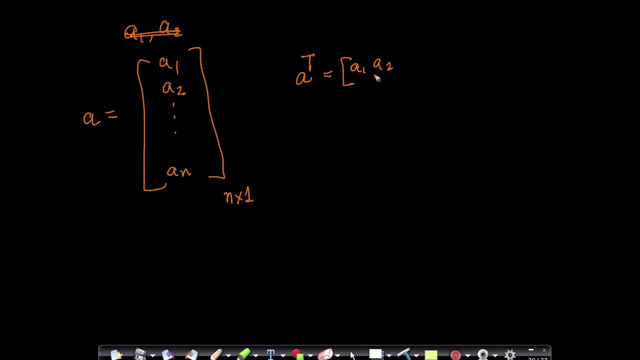 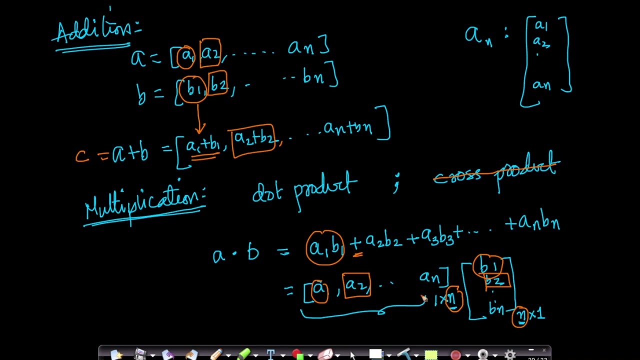 would immediately recognize this. A transpose is nothing but A1, A2, so on, so forth: A1.. So I can convert a column vector into a row vector by just taking an operator called transpose, and this becomes 1 cross N. So, going back to our previous example, what we have here, 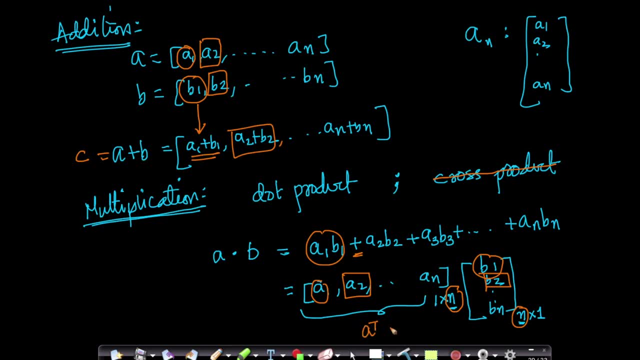 literally is nothing but A transpose multiplied by B, Right, So you can write A dot B as nothing but A transpose B. And what does it all boil down to? It boils down to summation of 1 to N. if A is an N-dimensional vector, A, i, B, i. 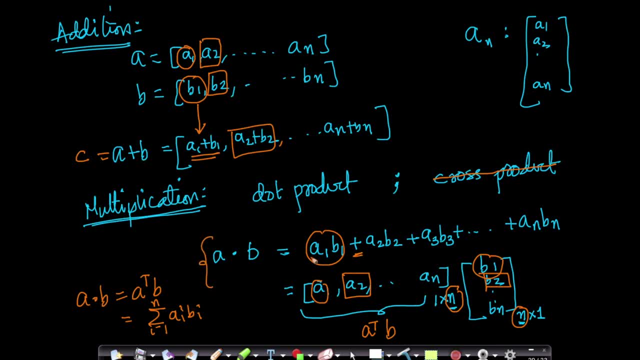 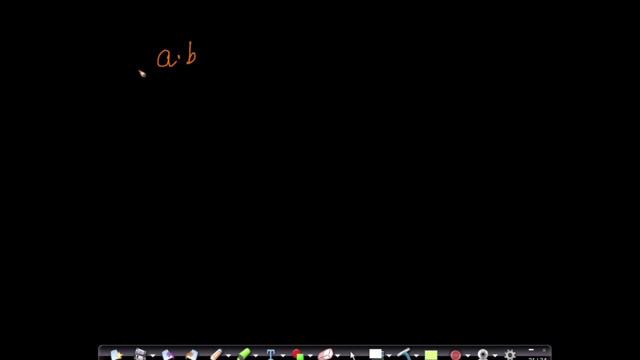 This is what a dot product is from a pure linear algebraic perspective. But now let us go and understand geometrically. what does A dot B mean? Because that is important. right, We have to connect geometry with linear algebra, Because if you do not connect it, 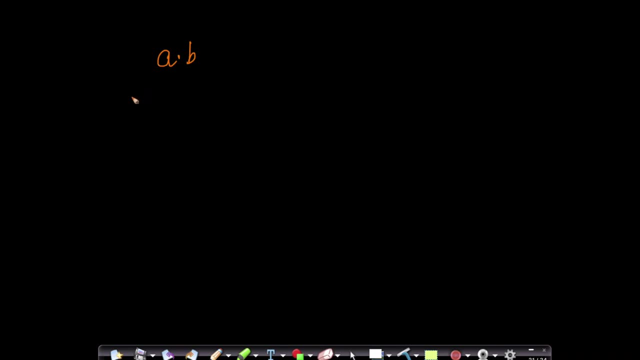 we do not understand what a dot product means in higher dimensional spaces, Because we are doing all of this linear algebraic exercise to understand geometry. So let us take, let us assume, we live in a two-dimensional space or we have a two-dimensional space. Let us assume I have a vector A and I have 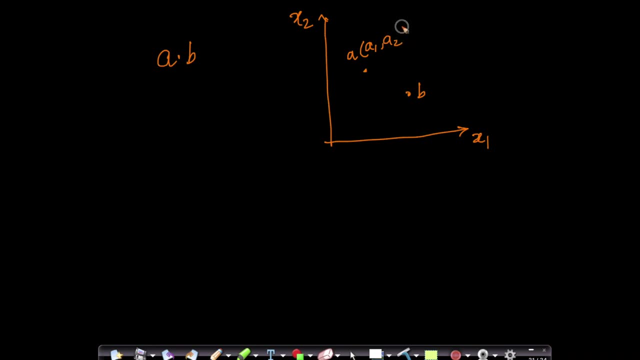 a vector B. Of course, A has two components: A1 and A2.. B also has two components: B1 and B2.. Right Now, when we have these two components, this is your vector A. right, This is your vector B. 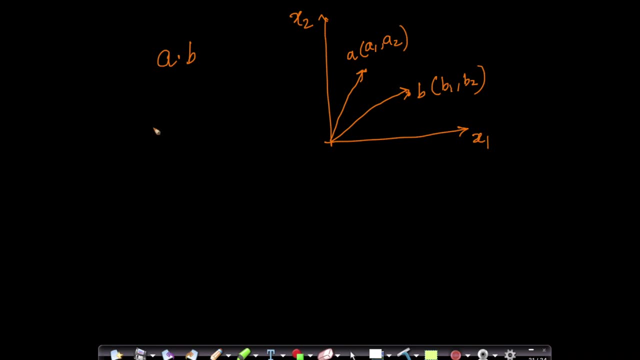 Now, what does A dot B represent geometrically? A dot B represents. A dot B can be written, as I will explain what each of them mean. Okay, let us assume the angle between A and B is theta and the length of A. So this is nothing but the length of A. 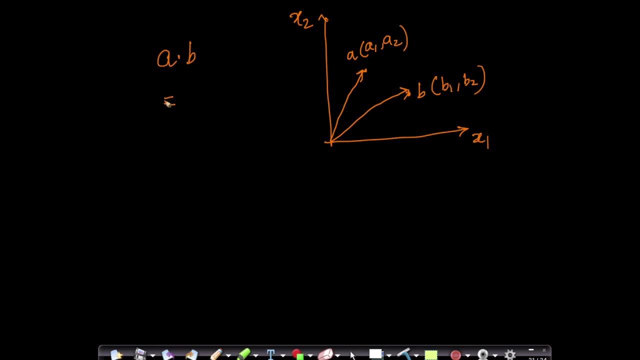 A dot B represents A dot B can be written as I will explain what each of them mean. Okay, let us assume the angle between A and B is theta and the length of A. So this is nothing but the length of A. 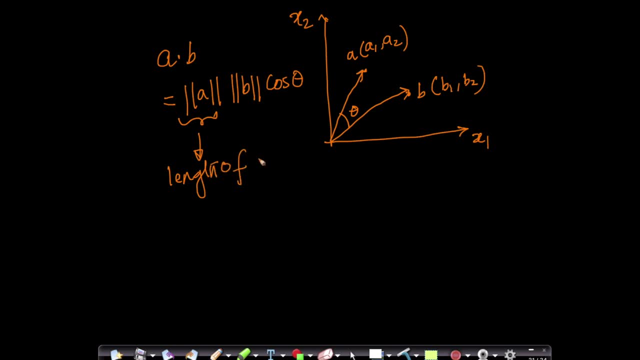 Okay, length of vector A. and this is your origin, right? So length of A is nothing but distance from distance of A from origin. Similarly, this is length of B, So length of a vector is represented with two dashes surrounding it. 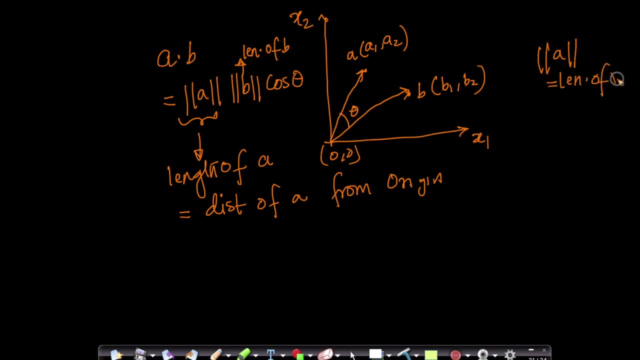 Okay, this is nothing but length of a vector. Okay, so what is what is A with two bars behind it? It is nothing but this length, this length. Let me just highlight it for you: It is nothing but this length, and this length is nothing but B. 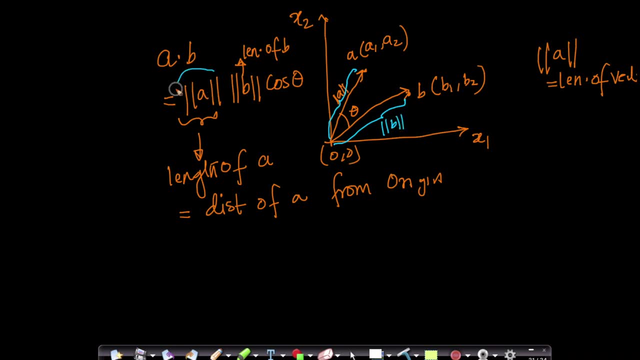 So A dot B is nothing but the length of A multiplied by length of B, multiplied by cos of the angle between them right Now. this is very useful. Now if somebody gives you two vectors as A1, A2.. How do you determine what is the angle between them right? 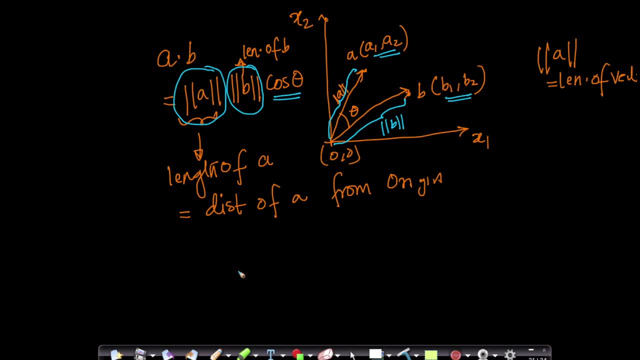 So let us quickly see that. So if somebody gave you A and B, what is? I can write A dot B as A1, B1 plus A2, B2, which is also equal to length of A length of B cos theta, which means theta is nothing. 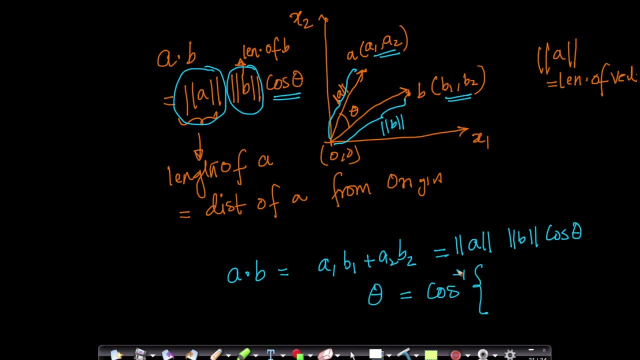 but cos inverse of. some people also call it arc cos cos inverse of A. So A1, B1 plus A2, B2, right divided by length of A and length of B, and we know that length of A, length of A is nothing but A1 square plus A2 square, under root. 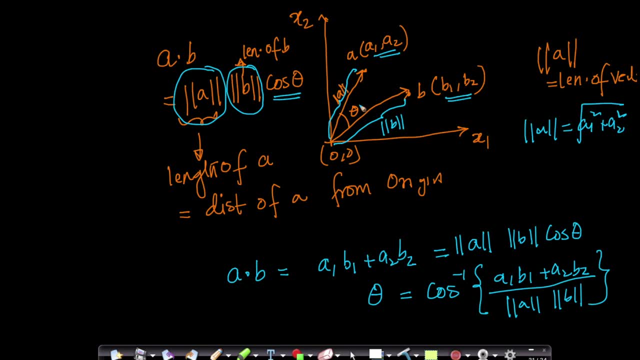 We saw this right distance of a distance of a point from an origin in one of the previous videos. So this is the length, length of a vector. So if somebody gives you two vectors, A and B, you can easily find the angle between both. 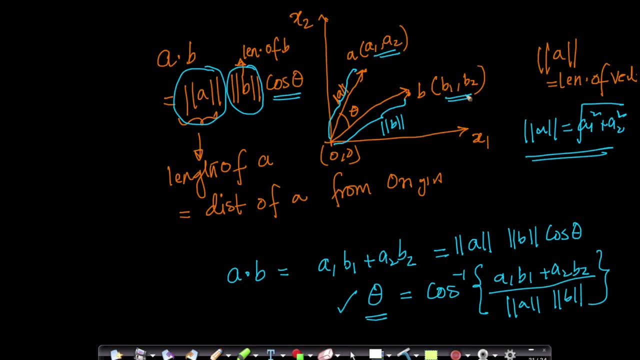 of them. If you just know the components A1, A2, B1, B2, right, I can still write. so basically I can write this A the length of A as A1 and A2.. So if you just give me the components of A1, A2, B1, B2, I can find the angle between. 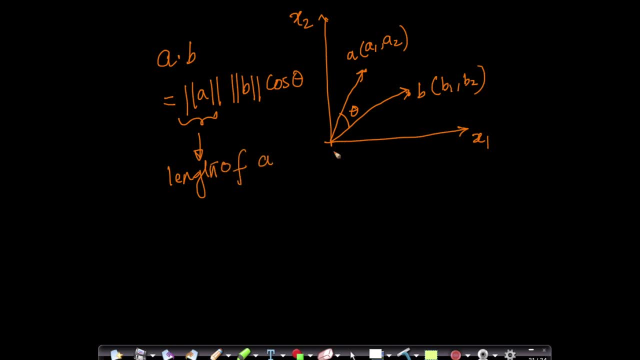 length of vector A, And this is your origin, right? So length of A is nothing but distance from distance of A from origin. Similarly, this is length of B, So length of a vector is represented with two dashes surrounding it. Okay, this is nothing but length of a vector. Okay, so what is A with two bars? 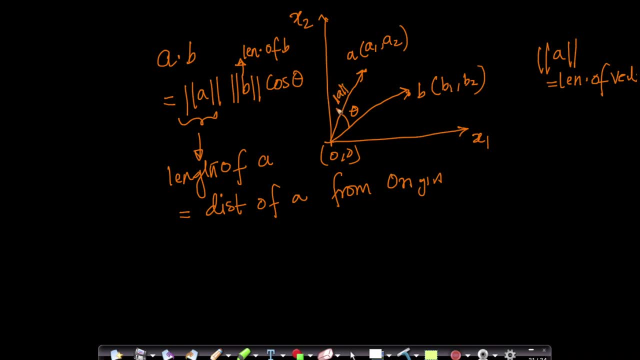 behind it. It is nothing but this length, this length. Let me just highlight it for you. It is nothing but this length and this length is nothing but b. So a dot b is nothing but the length of a multiplied by length of b multiplied. 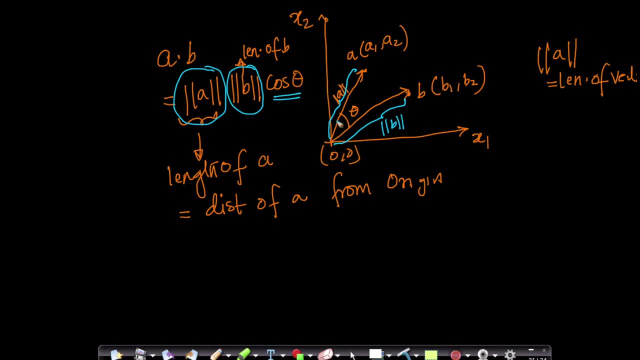 by cos of the angle between them right Now. this is very useful. Now, if somebody gives you two vectors as a1, a2, how do you determine what is the angle between them, right? So let us quickly see that. So if somebody gave you a and b, what is? I can write a dot b as a1, b1 plus a2, b2. 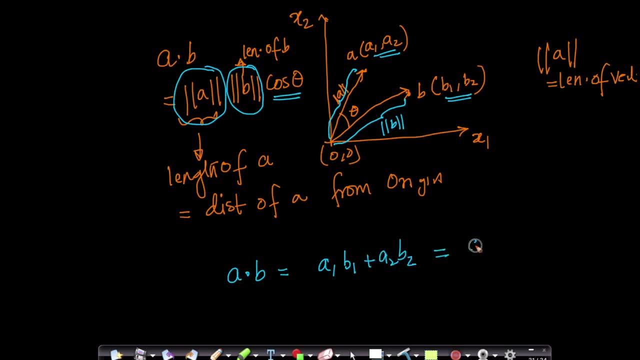 which is also equal to length of a length of b cos theta, which means theta is nothing but cos inverse of- some people also call it arc- cos cos inverse of a1, b1 plus a2, b2, right divided by. 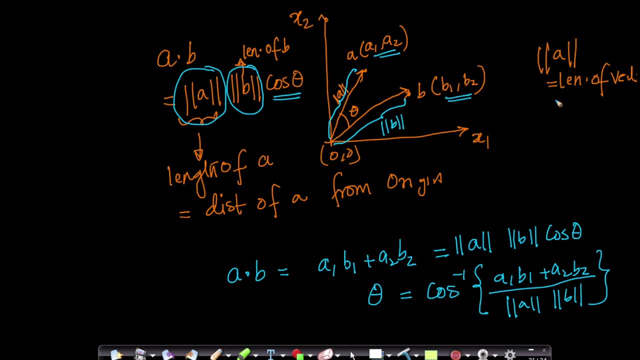 Length of a and length of b, and we know that length of a length of a is nothing but a1 square plus a2 square under root. We saw this right distance of a point from an origin in one of the previous videos. So this is the length of a vector. So if somebody gives you two vectors, a, 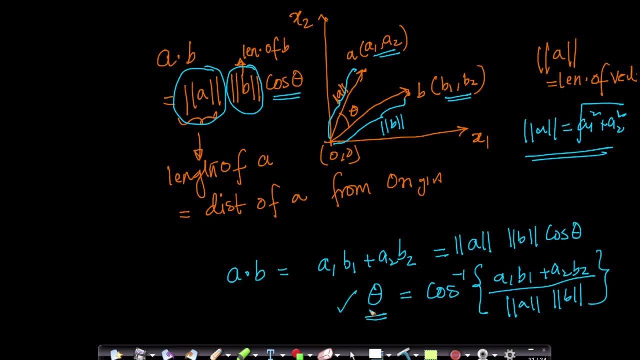 and b. you can easily find the angle between both of them if you just know the components a1, a2, b1, b2, right? So basically I can write this: a the length of a as a1 and a2.. So if you just give me, 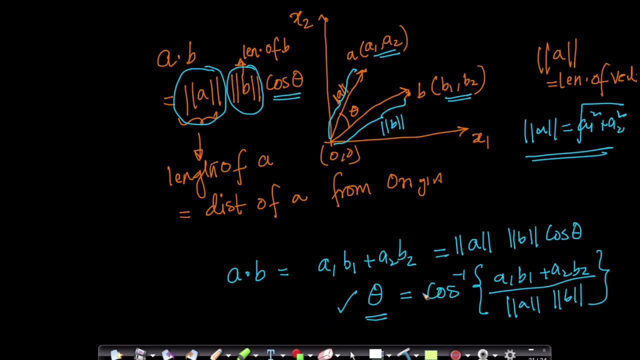 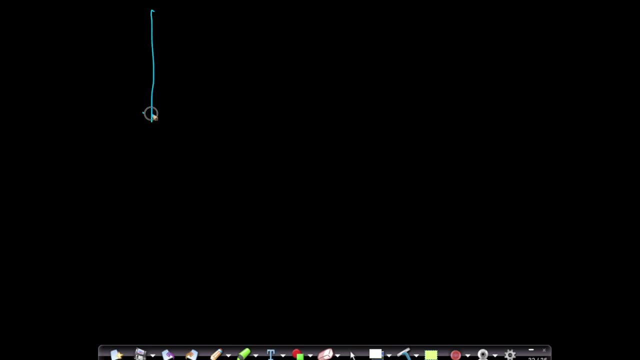 the components of a1, a2, b1, b2, I can find the angle between those two vectors. Now this takes us to an interesting idea: What if I have two vectors? Let us say I have two vectors, okay, I have a vector a here and I have a vector b here. Let us assume, 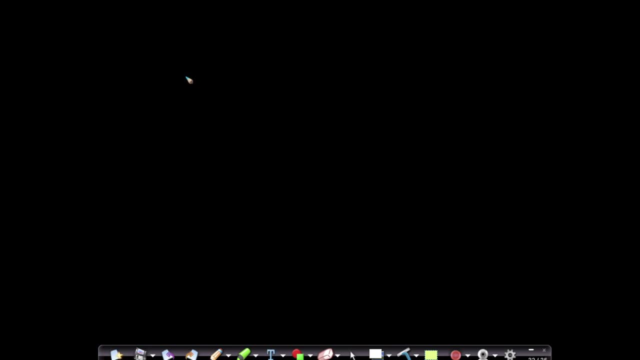 those two vectors. Now this takes us to an interesting idea. What if I have two vectors? Let us say I have two vectors, okay, I have a vector A here and I have a vector B here. Let us assume they are perpendicular to each other, which basically means the angle between: 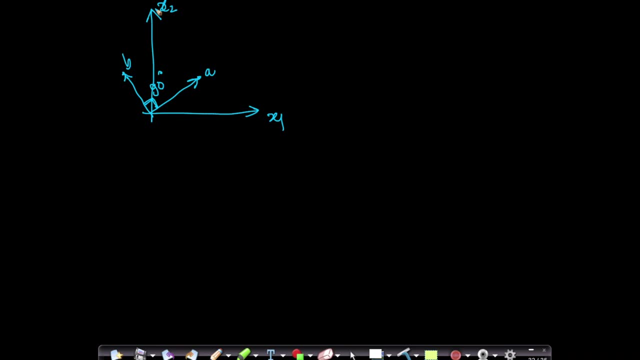 them is 90 degrees. Okay, let us assume this is x1 and this is x2, two dimensions, right? Your A is A1, A2, your B again is B1, B2.. Now the quick question is: what is now, if I know that A dot B, what will A dot B be? 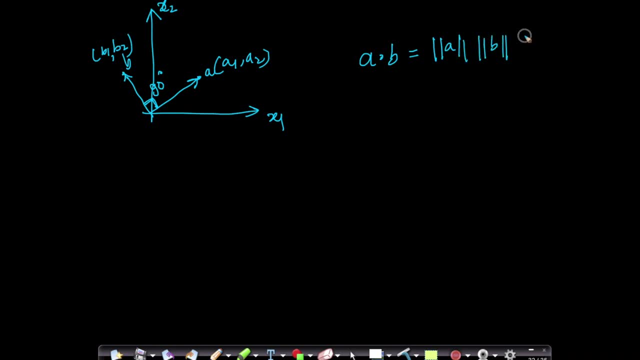 like: Okay, length of A length of B and cos of 90. And I know that cos of 90 is 90. And I know that cos of 90 is 90. So A dot B will be 0, because this is 0, right. 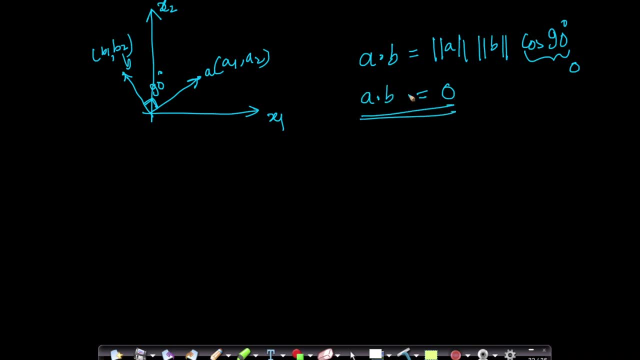 So if a dot product between two vectors is 0, we know that those two vectors are perpendicular to each other, right? So remember, this whole idea of angle between two vectors can be extended to any dimensions. Your A could be any dimensional vector- A1,, A2, it could lie in any dimensions it could. 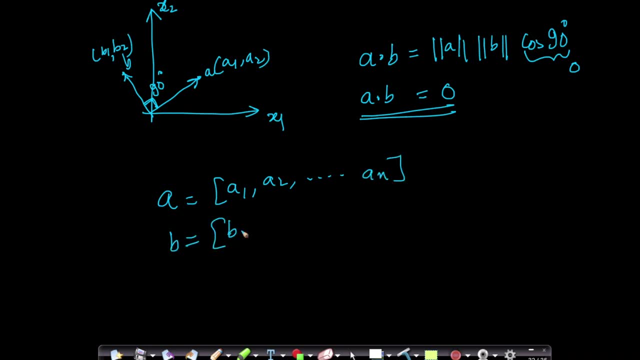 lie in an n-dimensional space. B2, yes, sir, B also. B also can exist in an n-dimensional space. It does not matter. Even though we cannot visualize anything more than 3D, your A and B could be in any dimensional. 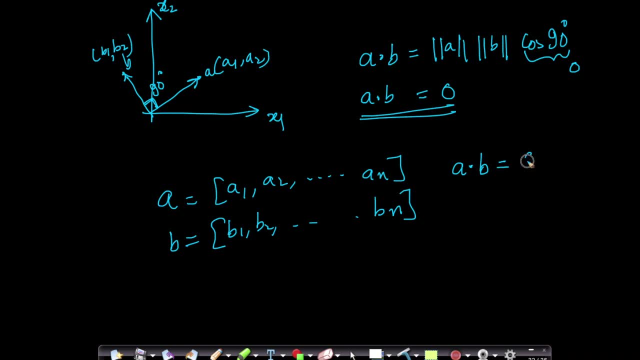 space. I could just compute A dot B, which will always be length of A and length of B, and cos theta right, which means I can compute the theta as cos inverse of A, i, B. i summation right by length of A and length of B. 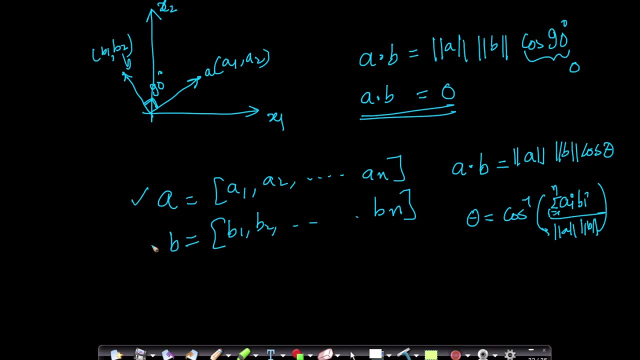 So if you give me two vectors in any dimensional space, I can compute the angle between those two vectors. I can compute the theta between A and B very, very easily, because what I have learnt in 2D, I am just extending it to n-dimensional space, right? 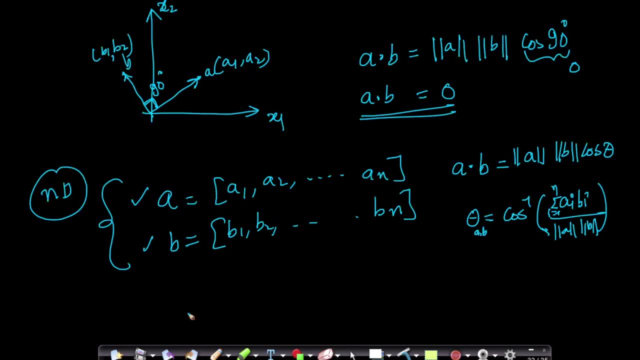 This is what I learnt in 2D, right? Whatever I learnt in 2D, I am just extending it to n-dimensional space. Similarly, if I have two vectors in n-dimensional space and if I compute A, dot, B, what is A? 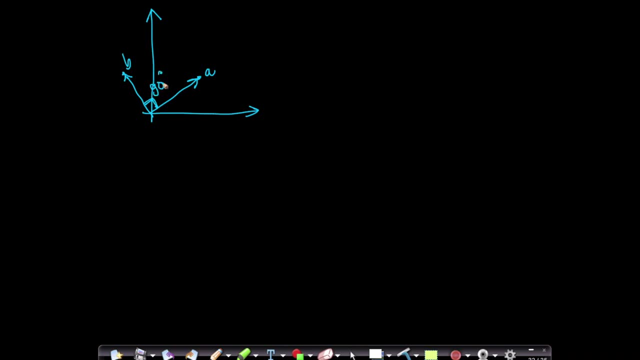 they are perpendicular to each other, which basically means the angle between them is 90 degrees. Let us assume this is x1 and this is x2, two dimensions, right? Your a is a1, a2.. Your b again is b1, b2.. Now the quick question is: what is now? if I know that a dot b, what? 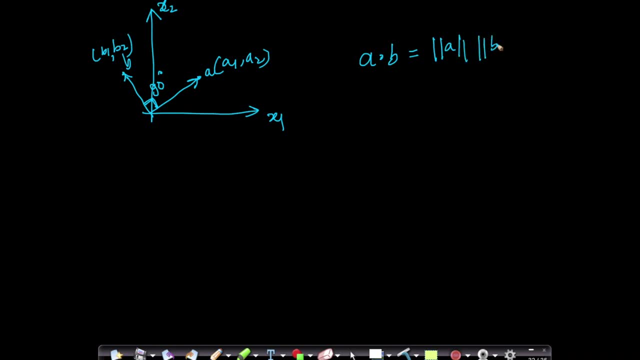 will a dot b be like: Okay, length of a length of b and cos of 90, and I know that cos of 90 is 0. So a dot b will be 0 because this is 0, right? So if a dot product between two, 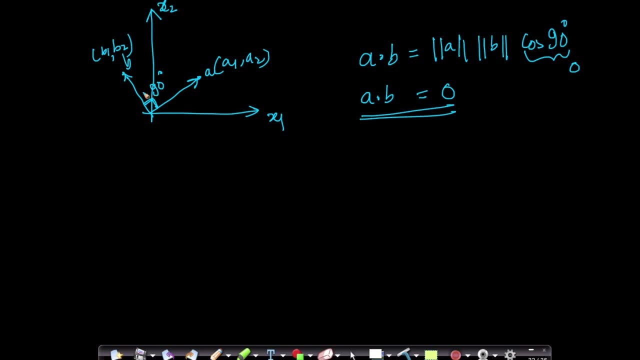 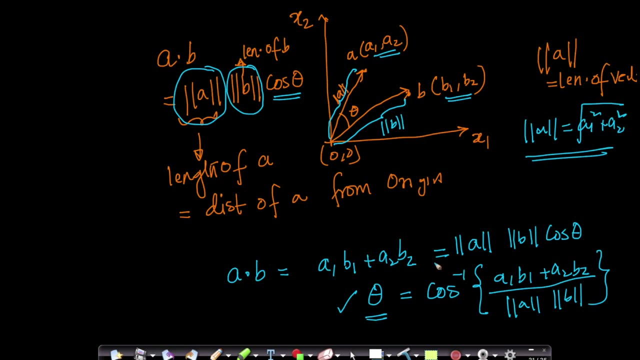 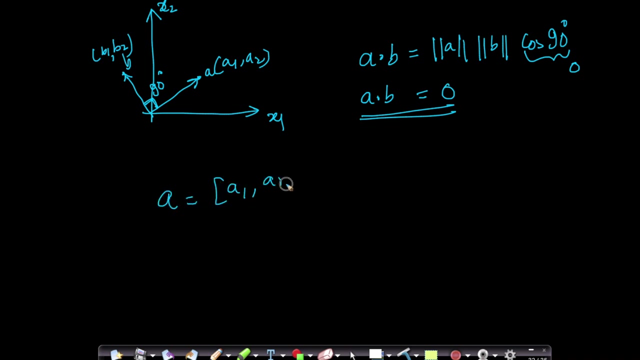 vectors is 0, we know that those two vectors are perpendicular to each other, right? So remember, this whole idea of angle between two vectors can be extended to any dimensions. Your a could be any dimensional vector: a1, a2.. It could lie in any dimensions It could. 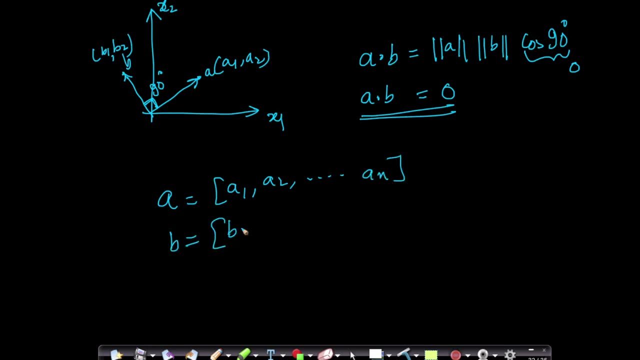 lie in an n-dimensional space- b2, where a is a1, a2, b2,, a1, a2, b2, a1, a2, a1, a2, a2, b2, b2, b also can exist in an n-dimensional space. It does not matter, Even though we. 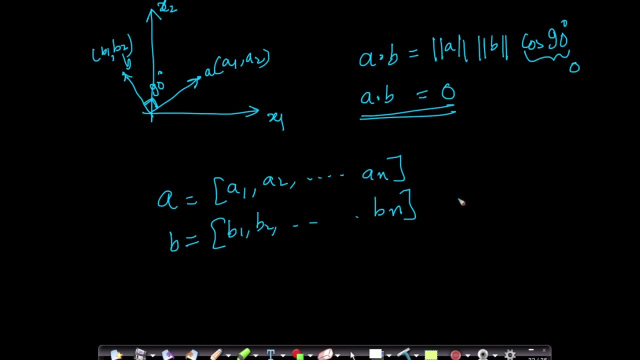 cannot visualize anything more than 3D. Your a and b could be in any dimensional space. I could just compute a dot b, which will always be length of a and length b and cos theta right, Which means I can compute the theta as cos inverse of a, a, i, b. i summation right. 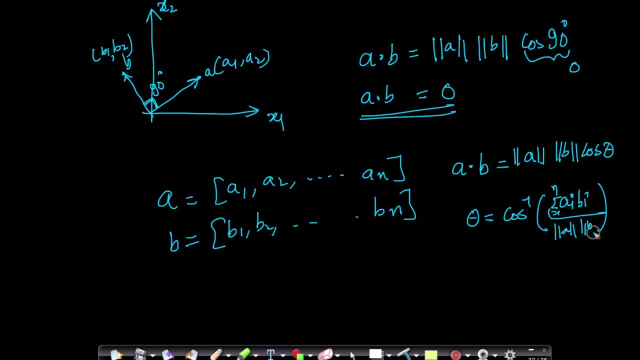 by length of A and length of B. So if you give me two vectors in any dimensional space, I can compute the angle between those two vectors. I can compute the theta between A and B very, very easily, Because what I have learned in 2D, I am just extending it to n dimensional space. 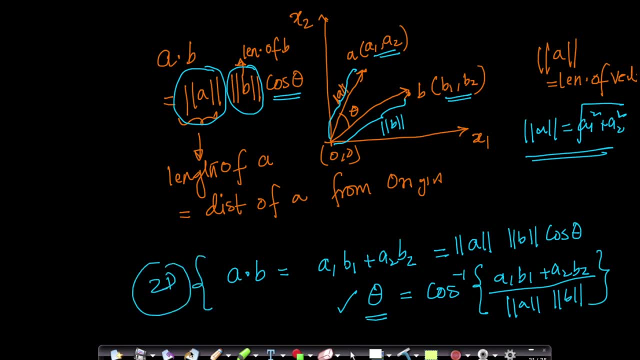 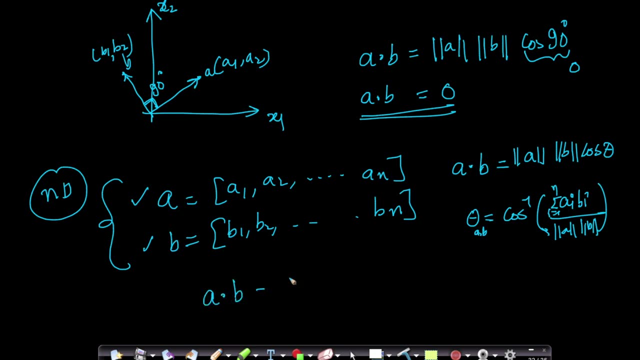 This is what I learned in 2D, right? Whatever I learned in 2D, I am just extending it to n dimensional space. Similarly, if I have two vectors in n dimensional space and if I compute A dot B, what is A dot B? A dot B is nothing but summation over. i equals to 1 to n. A, i, B, i. 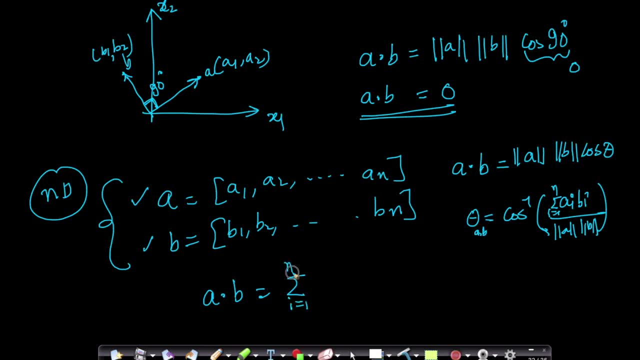 dot B. A, dot B is nothing but summation over. I equals to 1, to n, A, i, B, i. If that turns out to be 0, I know whatever dimension, the space that A and B could lie. All that this implies that A is perpendicular to B, right. 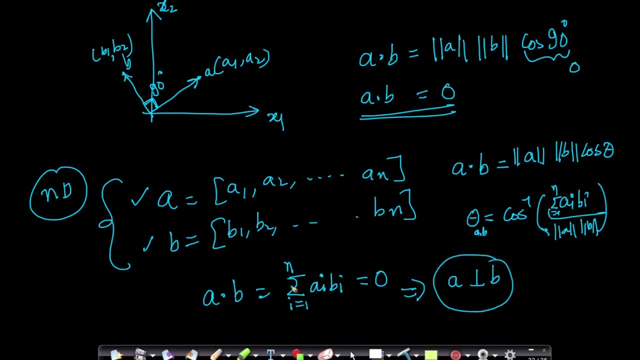 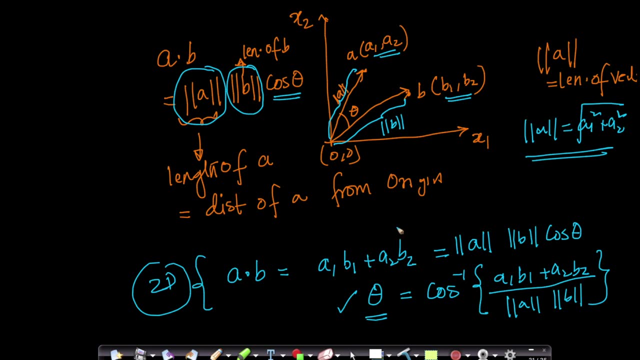 I do not care whether you are operating in 2D, 3D or n-D. This is the beauty of linear algebra. In linear, algebra and coordinate geometry are very nicely connected through relationships like this, and whatever we learn in 2D we can easily extend it to n-D. 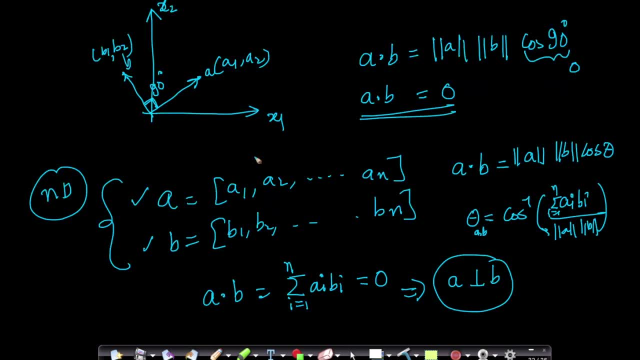 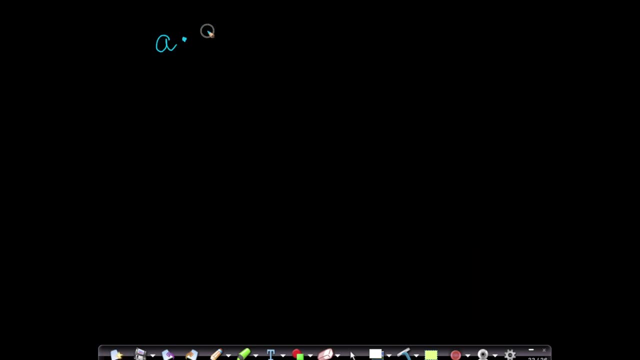 Because vectors could be of 2D, 3D or any dimensions and all the geometric intuition that we are learning from 2D. we can extend it to any dimensional space. Now the next question is: what about A dot A? What if I multiply, I do a dot product of A with A. 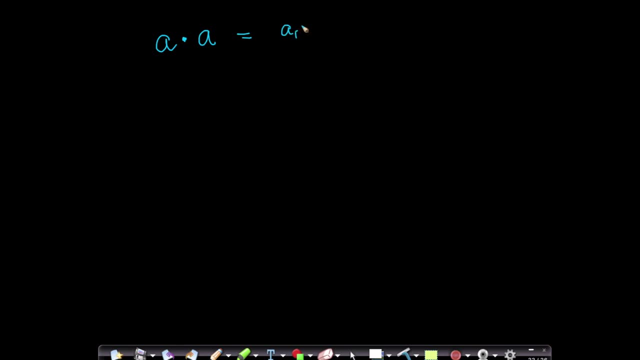 What does A dot A actually mean? It basically means A1 into A1 plus A2 into A2, so on, so forth. A n into A n, and this is nothing but A1 square Plus A2 square. so on, so forth. A n square, and this is nothing but the distance of A. 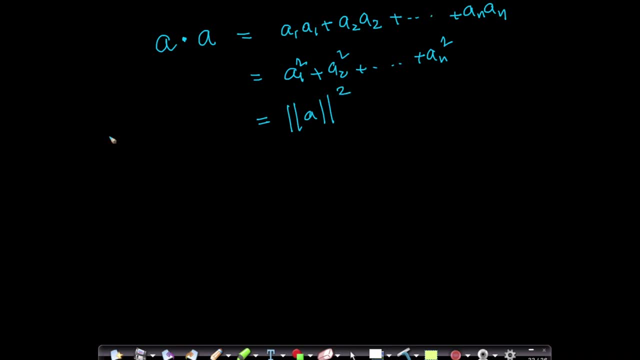 from origin squared right. We know that given any point A, given any point A, its distance from origin is nothing but A1 square plus A2 square plus, so on, so forth. A n square under root right. We know that the distance from origin D can be written as this: and when we do A, dot A. 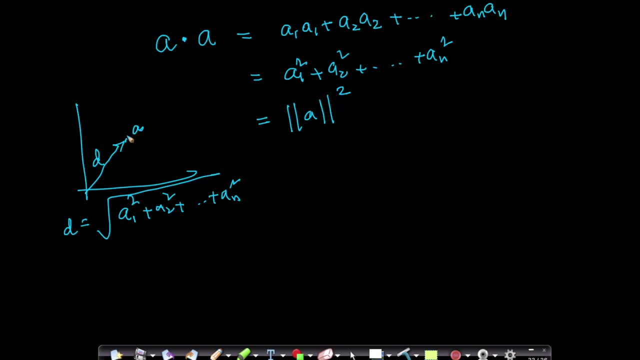 get is basically square of the distance of that vector A from origin, and this could. this is in any dimensional space. the theory still just holds. good, that is the beauty of it. So what we have done is we have written dot product in 2D right. 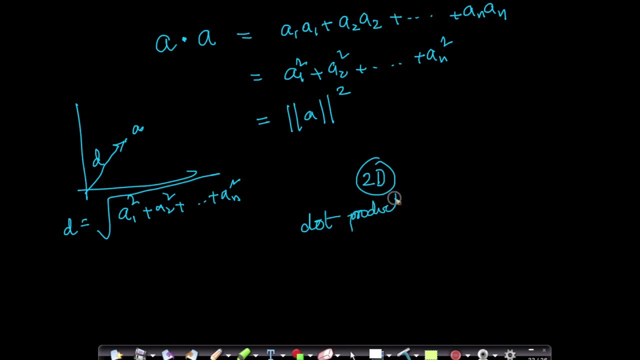 We have written about dot product in 2D right and we have understood it geometrically as angles between points, and we are extending the same idea to n dimensions because dot product can be generalized to n dimensions And from that generalization we are understanding the n dimensional geometry without being able. to visualize it. That is the super duper power of linear algebra. 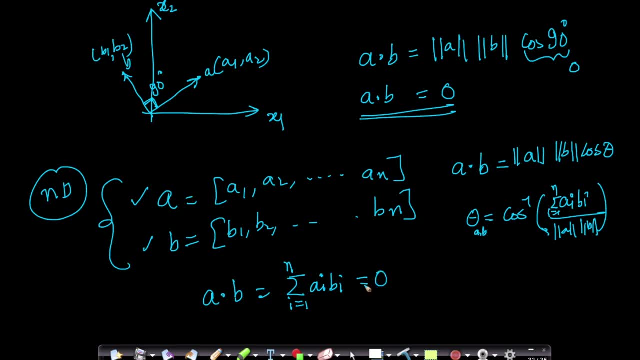 If that turns out to be 0, I know, whatever dimension, the space that A and B could lie, All that this implies that A is perpendicular to B, right? I do not care whether you are operating in 2D, 3D or n? D. This is the beauty of linear algebra: In linear algebra and coordinate. 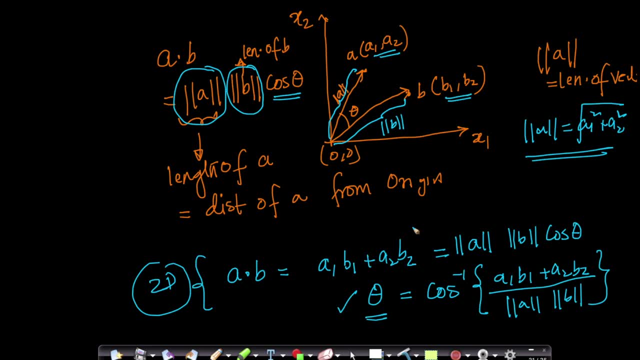 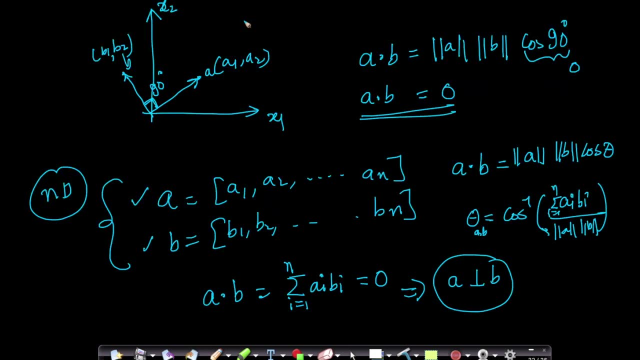 geometry are very nicely connected through relationships like this. And whatever we learn in 2D, we can easily extend it to n? D, because vectors could be of 2D, 3D or any dimensions. And all the geometric intuition that we are learning from 2D, we can extend it to any. 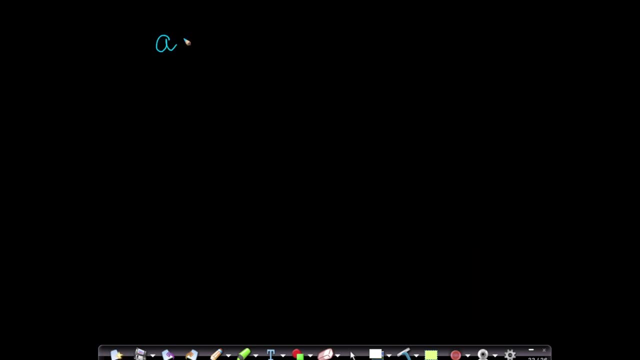 dimensional space. Now the next question is: what about A dot A? What if I multiply, I do a dot product of A with A. What does A dot A actually mean? It basically means A1 into A1 plus A2 into. 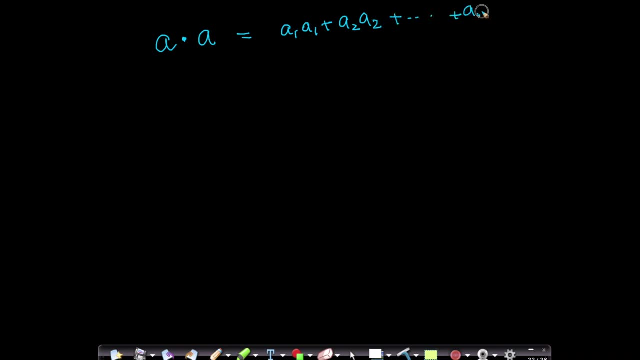 A2, so on, so forth. An into An, And this is nothing but A1 square plus A2 square, so on, so forth. An square, And this is nothing but the distance of A from origin, squared right. We know that, given any point A, given any point A, 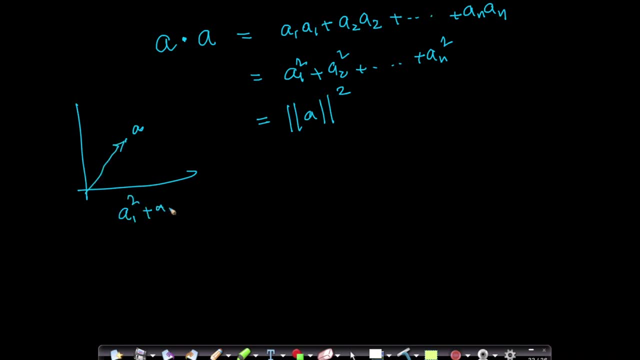 its distance from origin is nothing but A1 square plus A2 square plus so on, so forth An square under root right. We know that the distance from origin, D is can be written as this, And when we do A dot A, what we get is basically square of the distance. 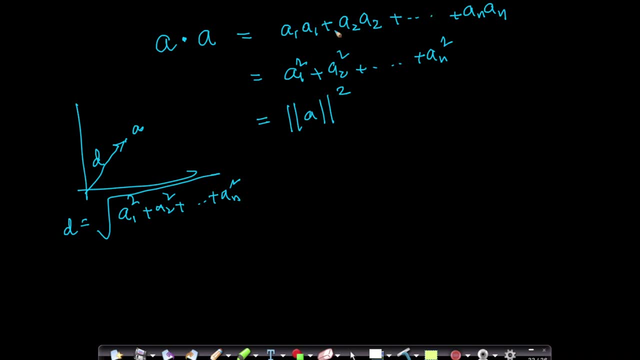 of that vector A from origin, And this could. this is in any dimensional space. The theory still just holds good, That is the beauty of it. So what we have done is we have written dot product in 2D. right, We have written about dot product in 2D. 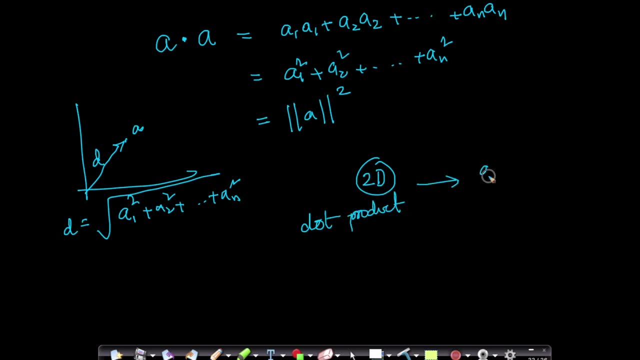 right And we have understood it geometrically as angles between points. And we are extending the same idea to n dimensions, because dot product can be generalized to n dimensions And from that generalization we are understanding the n dimensional geometry without being able to. visualize it. That is the super duper power of linear algebra.